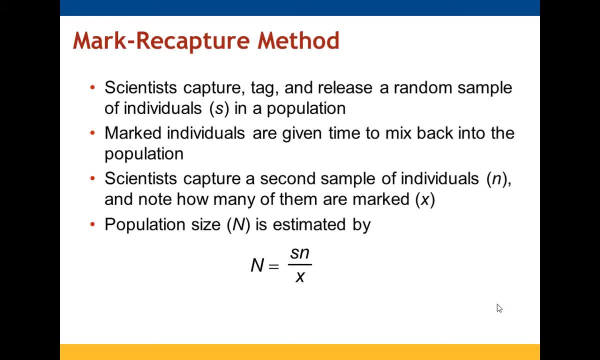 one right now. So what scientists will do is they will capture, they will tag and then they will release some of the individuals present in the population. They will give those individuals an opportunity to mix back in and then they will capture a second set of a second set sample of. 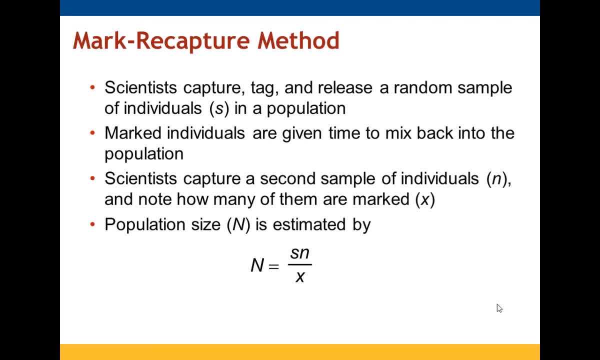 individuals and identify how they are doing, And then they will capture a second set of a second sample of individuals and identify how many of them are marked previously, And then they will use that information to estimate population size by taking the product of the number of individuals. 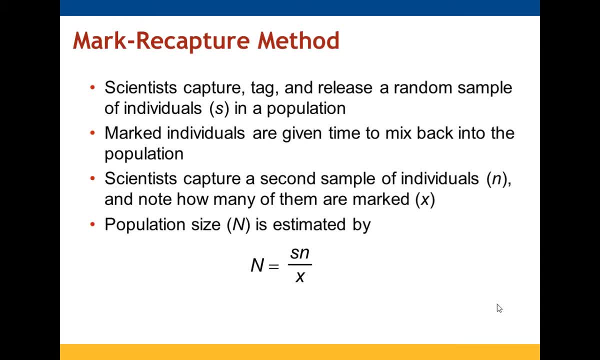 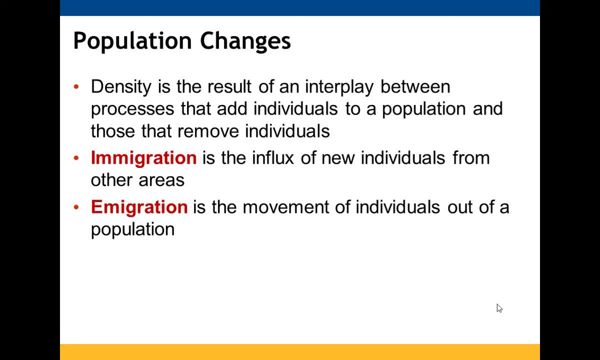 in the initial sample and the number of individuals in the second sample and dividing that product by the number that were marked. So density is going to kind of be an interplay between when individuals are added to populations and when individuals are removed And there's a 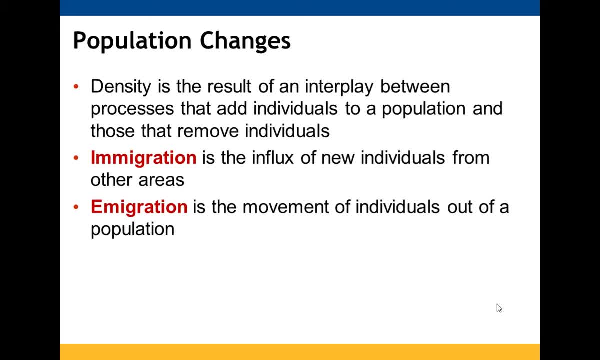 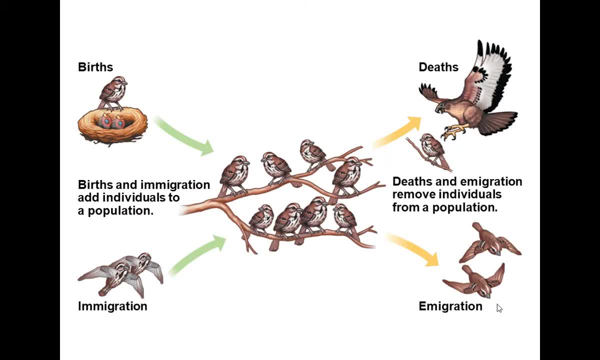 couple ways that can happen. It can happen from immigration and it can happen from emigration. Immigration and new individuals enter, Emigration, individuals move out. It can also happen from birth and from death. So birth and immigration will add individuals to your population, while 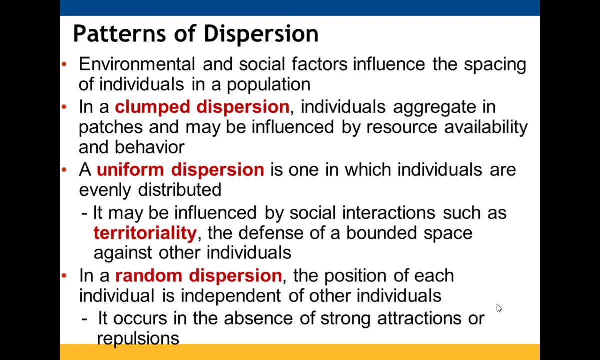 death and immigration will remove them. So we talked about dispersion patterns a little bit earlier. Environmental and social factors will influence these. In clumped dispersion we will have individuals kind of grouped together in, you know, in groups of individuals. So we're going to 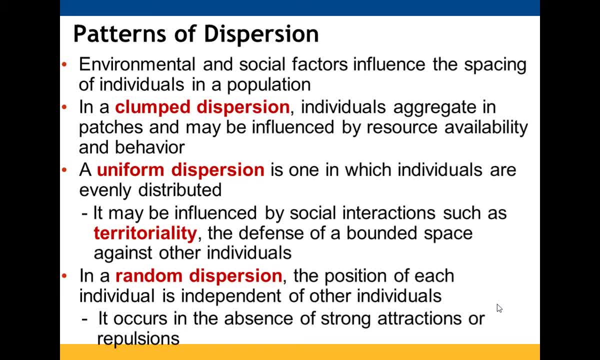 step involve individuals within different groups. Information, sure fact, check Again, it's not just a place that体 quoi. an information space less the Territory acesso, a portico of the location of that individual is coming, divided equally throughout that area can be. 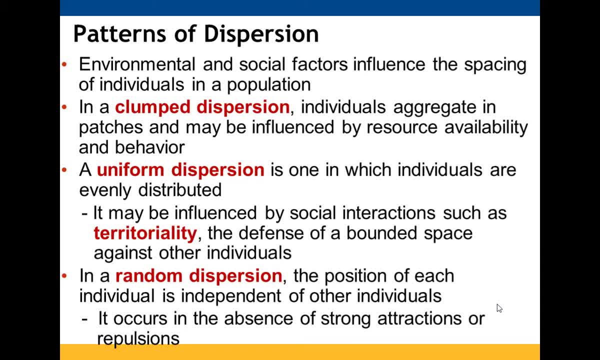 That tells Regitionally would mean that individuals are going to enter school have barriers within that area, not allally Every individual in there as well. And here's just a little bit of an example of how it can be used. It's pretty easy to take over. 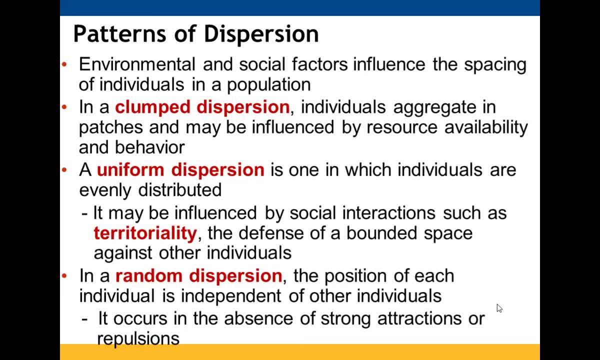 So the data is organized in there. Yeah, you can check that data and if there is a pattern there, every body is found is truly happenstance. Each individual is independent of the other. There's nothing pushing them towards one another and there's nothing pushing them away from one another. 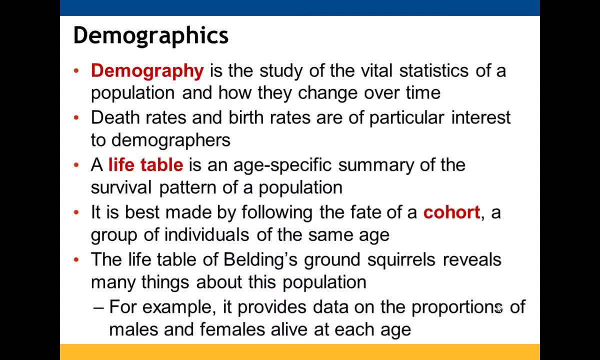 So there you see clumped, uniform and random Demographics is looking at statistics for a population and seeing how they are going through changes over time. Death rates and birth rates are definitely ones that we tend to look at. A life table shows us survival patterns by age. 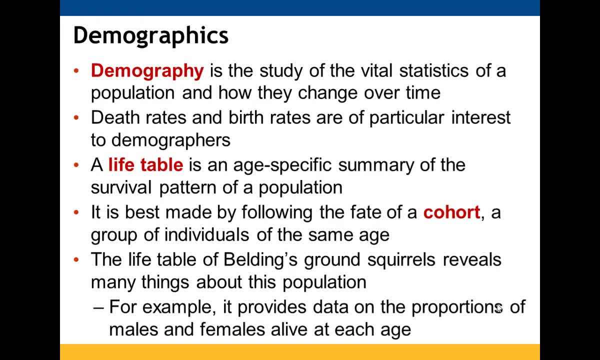 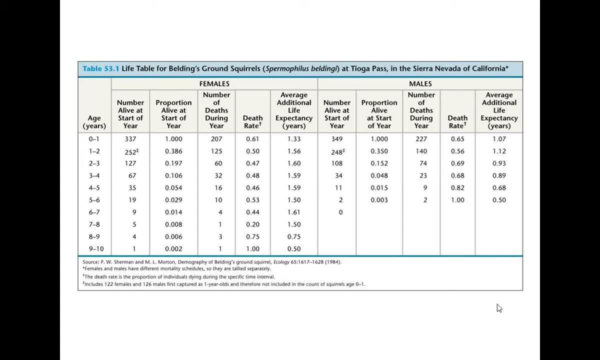 We tend to look at it in terms of cohorts, And so we're going to look at beldings, browns, squirrels, And if you look at this particular table, you will see that there are roughly the same number of females as males, from zero to one, but that the males tend to pass away a little bit earlier. The 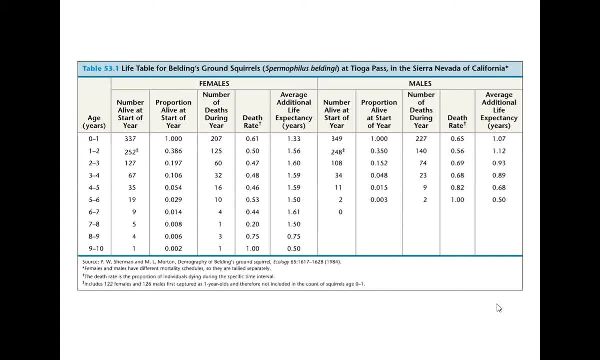 last male in this particular table from the day before was a male, And so we're going to look at the data that was collected- lived between five and six years, while the females lived up to nine to ten years. But you can kind of see how the number that are alive at the beginning of each 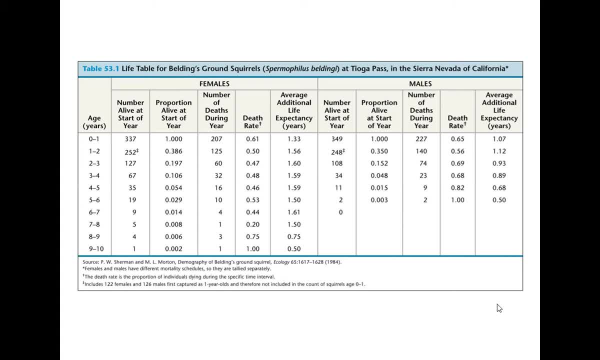 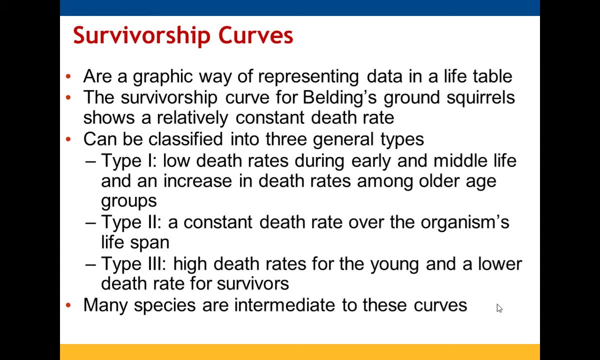 year are decreasing over those periods of time. Survivorship curves are a way we can look at that data that's present in a life table And what we see for the belding ground squirrels is that it's a pretty constant death rate. So there's basically three. 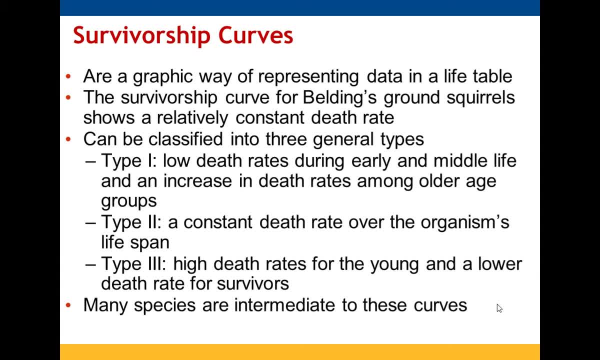 There's three ways we could look at survivorship curves from life tables. We could have a type two, which is what we see with the belding ground squirrels: a constant death rate over the organism's lifespan. A type one is when we see fairly low death rates in early and middle ages. 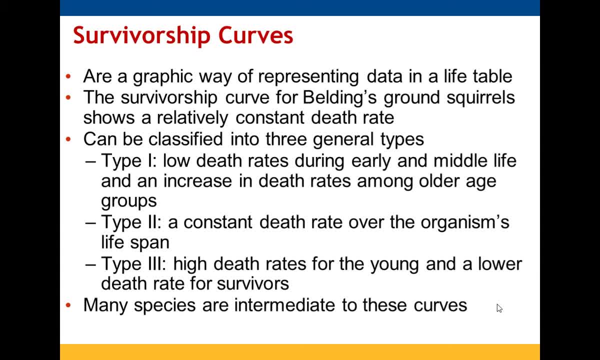 an increase among older ages. That would be what we see typically with humans. And then type three: you have really high death rates for the young and you have a much lower death rate for the survivors, And again there's going to be very high death rates for the young. And then type three: 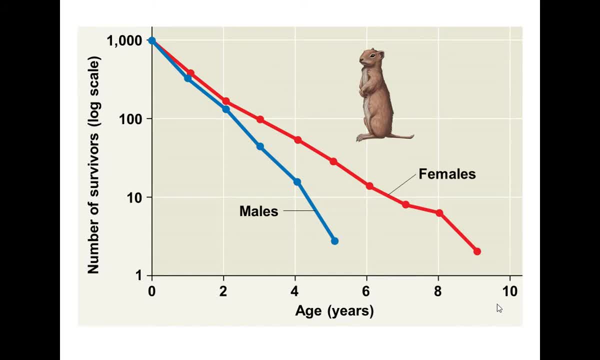 you have very high death rates for the older ages, And again there's going to be very high death rates for the younger ages, And again there's going to be very high death rates for the younger ages between these. So there you can see the belding squirrels, how the females are going to. 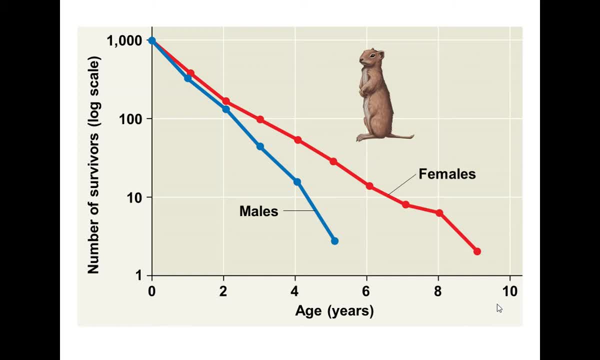 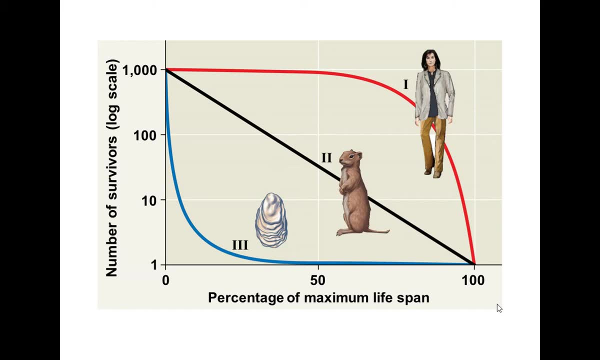 they didn't drop off as rapidly as the males, They were able to live for a little bit longer period of time. And then there's the type one, type two and type three survivor ship curves, one being human, two being the squirrels and three being a mollusk. I believe Sorry. 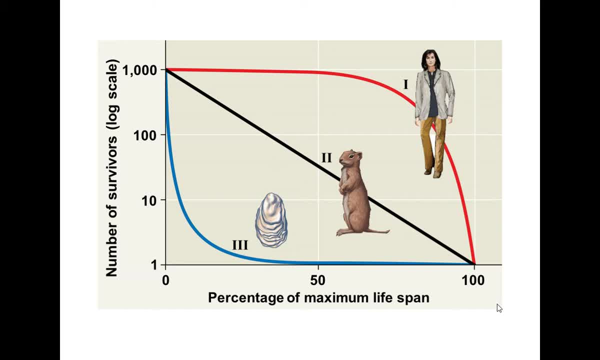 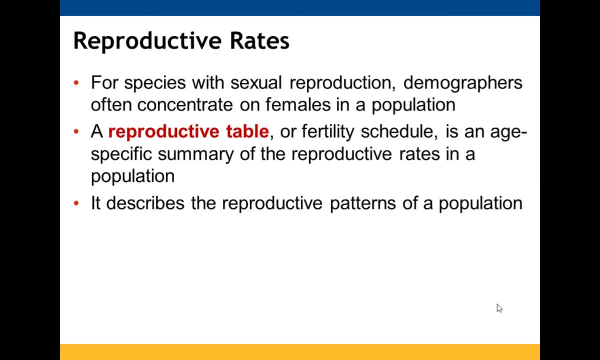 I didn't look it up again, But again an aquatic animal. Reproductive rates. Females are going to play a key role in examining reproductive rates, since they are the ones that either carry or provided the egg or embryo that was able to produce the offspring. 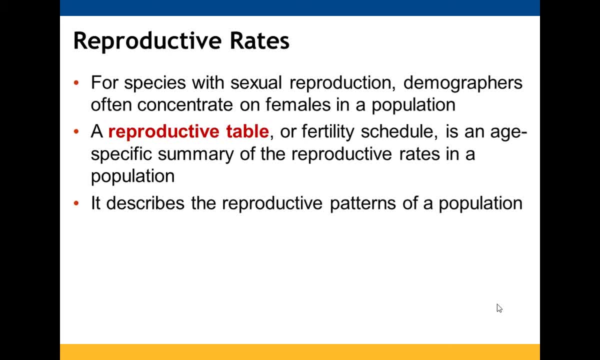 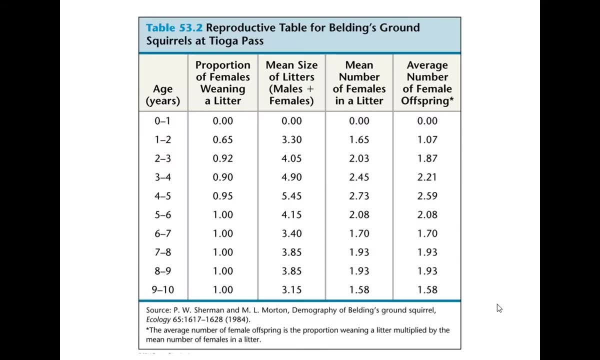 Reproductive table gives us age-specific summaries of those reproductive rates- When were they able to reproduce and what ages- And it is able to describe the reproductive patterns present in that population. So for the belding's ground squirrels we see that initially, from zero to one years of age, they were not weaning litters. 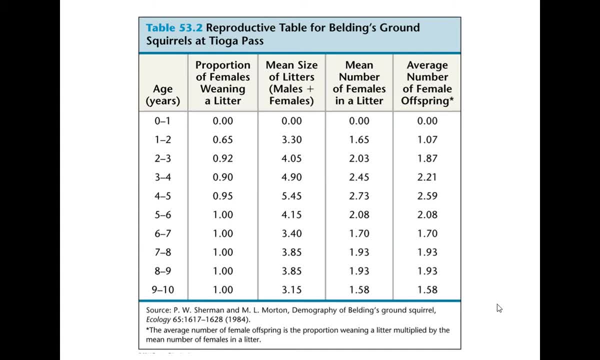 But then, pretty much after that, one to two- over half- were weaning litters And 90% or more were weaning litters between two and five years of age. And then, once we got to that point, all individuals that were still alive- granted, there weren't as many females as what we saw previously- were weaning litters. 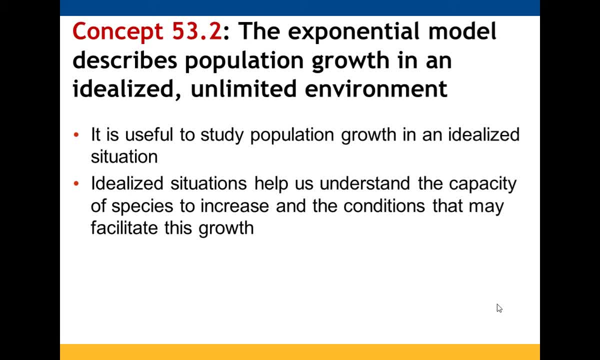 So we're going to look at two types of models. Exponential model is the first one, And this is looking at things basically in fantasy land, studying population growth in an idealized situation. It's helping us to understand capacity of species to be able to increase and what conditions might help them be able to increase exponentially. 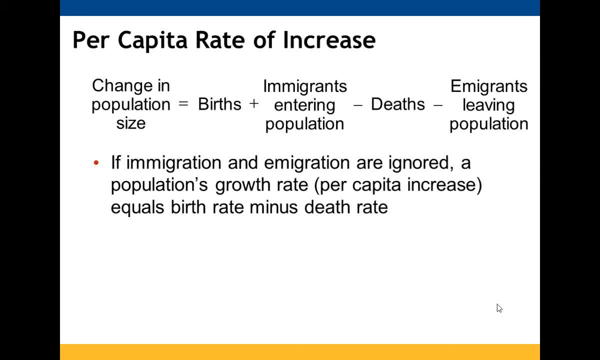 So if we are wanting to look at changes in population size over periods of time, we would want to account for the births and the immigration and take away from that the number of deaths and the number of emigrants. If we ignore the immigrants and the emigrants, basically it would be birth rate minus death rate. 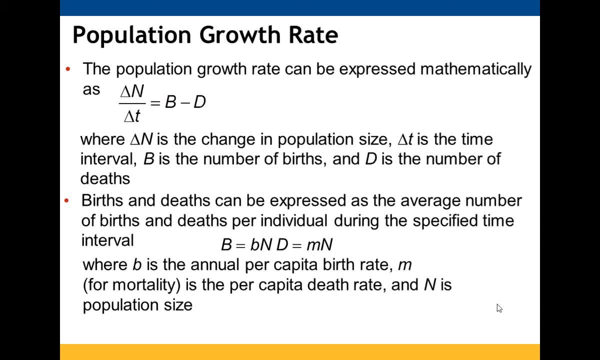 So if we wanted to focus on that, just looking at birth rate minus death rate, assuming that the immigration and emigration aren't going to play a huge role, our population growth rate would just be the difference between those To determine the value of B and D. we aren't going to count up again every six months. 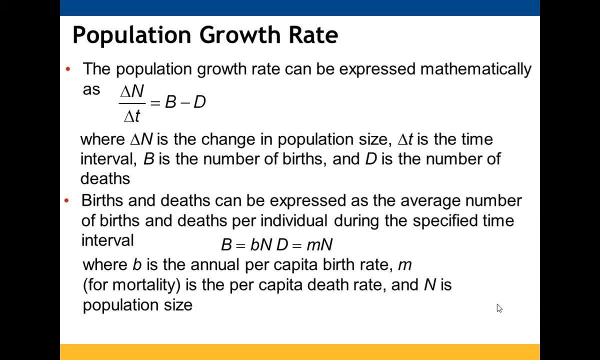 We're going to count up every single individual that's present in a population. We determine the average number of births and deaths per individual and multiply it by the population size that's present to get the birth and the number for births and the number for deaths. 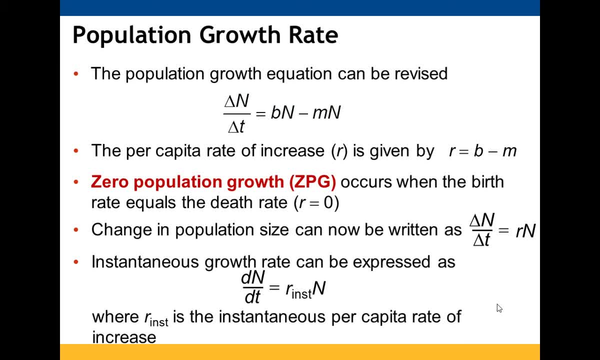 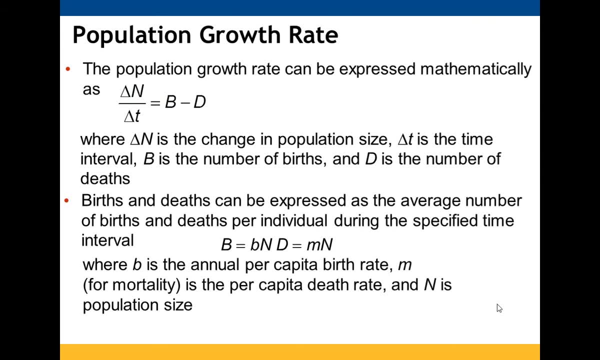 So if we wanted to revise this particular value, make sure I got this right- Yep, So if we were going to revise it. so you see how we said that the population number of births is going to be your birth rate over the year times the number of your population. 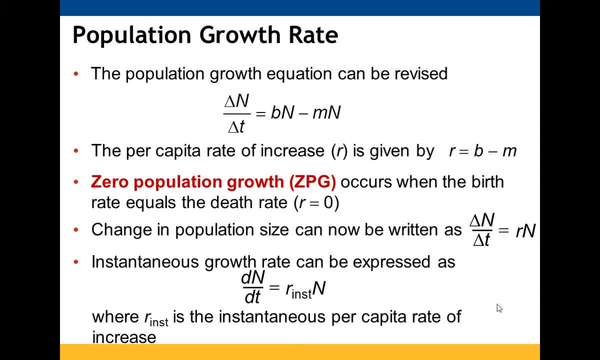 So that's just substituting in B and for big B and M and for big D. We can then determine what the rate of increase would be, because delta N over delta T would basically be that rate of increase, And since they both have a value of N, that would just be. 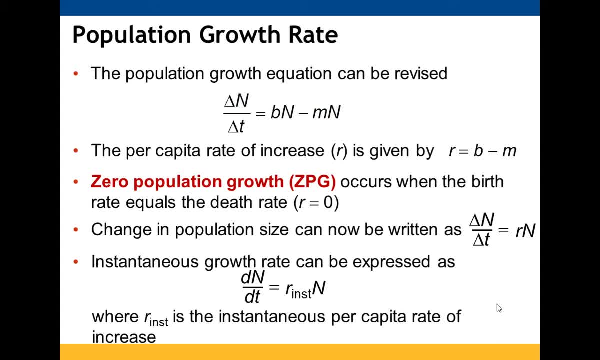 B minus M. Zero population growth is when your birth rate and your death rate are the same, So you didn't have an increase on one side or the other, And if that is the case, we could use that to find instantaneous growth rate. 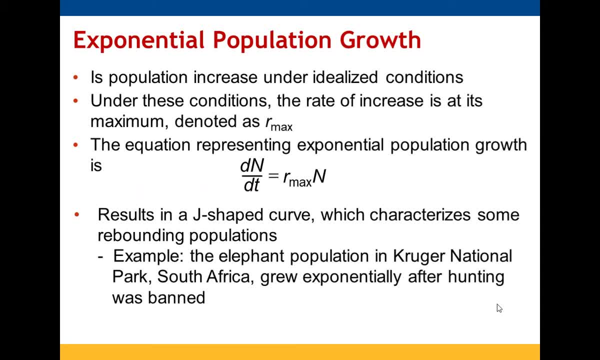 Exponential population growth rate again is idealized circumstances, And so this is when the increase is maximized as much as possible. It's going to result in a J-shaped curve. We do see this in some populations That are rebounding because there have been changes in their surroundings that have allowed them to grow without any restrictions. 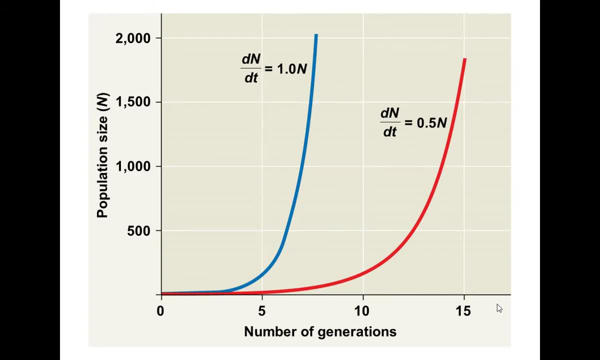 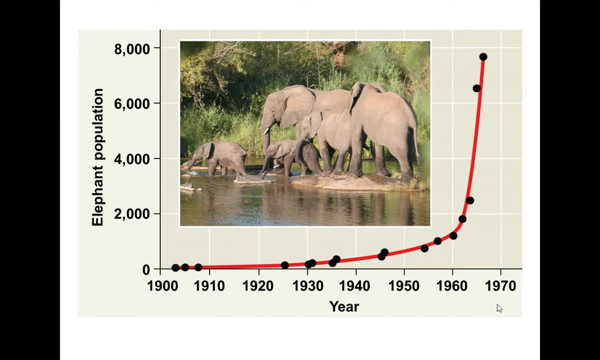 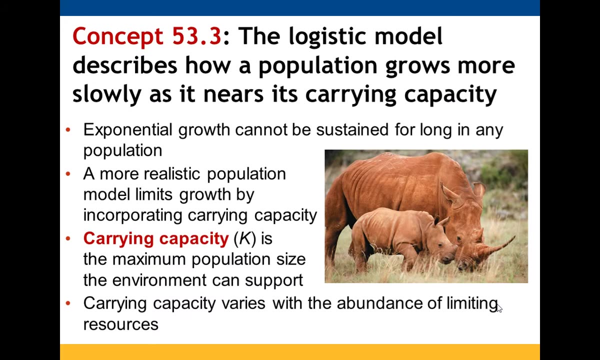 So we can see kind of there the letter J that we're referring to, with the exponential growth curve. And there's the elephants that were no longer being hunted, So they were able to grow quite quickly and the population increased dramatically. The logistic model is a little bit more realistic. 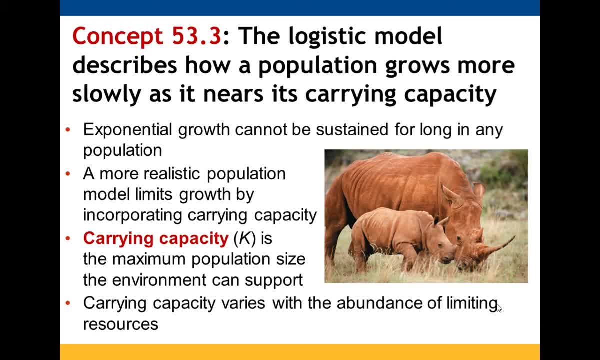 It's not absolute Um, but It basically shows how the population will grow until it's getting closer to its carrying capacity Um. the carrying capacity, which we're going to refer to as K, is going to be dependent on what resources are available in the environment. 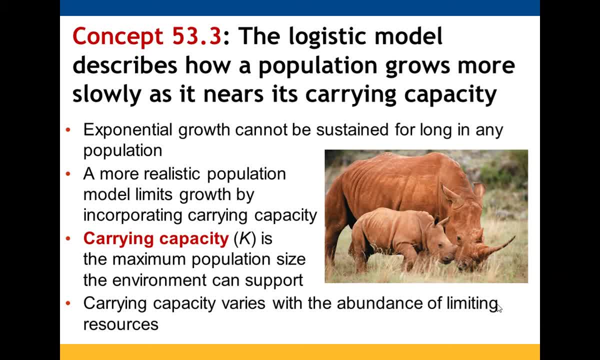 Um that's going to limit how many individuals within that um can live within that population. So the exponential growth um is again not going to be able to be sustained for an extended period of time. Um accounting: It's a little bit more realistic and that's where carrying capacity is going to come into play. 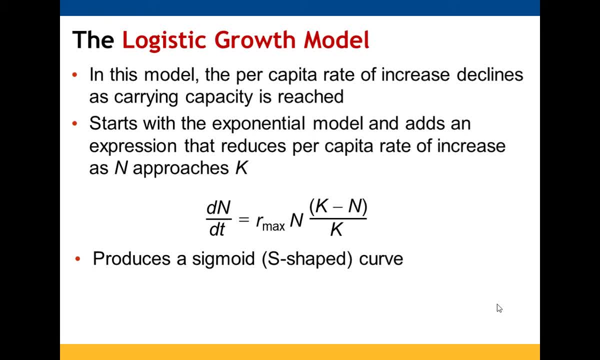 So with the logistic growth model, the rate of increase is going to decrease as you're carrying capacity is getting closer to it. So if we look at that exponential model and we account for the fact that we're going to slow down as we get closer to that carrying capacity, 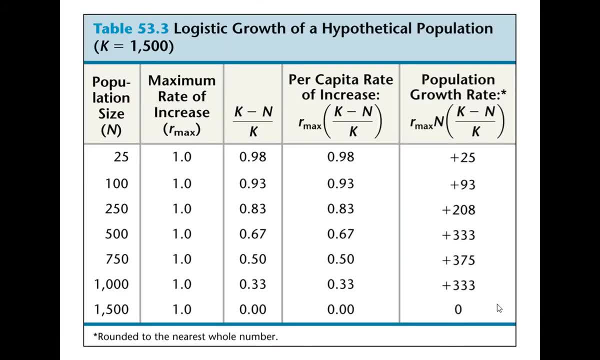 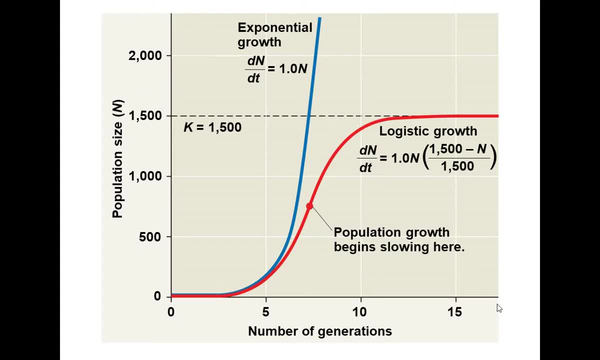 Um, we would generate a Sigma curve, an s-shaped graph, okay, um, so there's some data kind of showing you what those changes are going to look like, and that's more of a graphical representation. you can see the exponential graph, exponential growth in blue, the logistic growth in red, that, as we start to get closer to that. 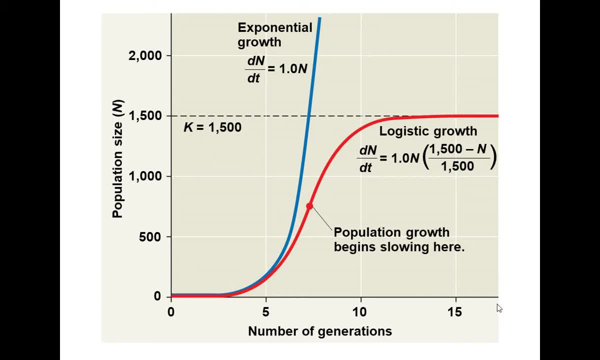 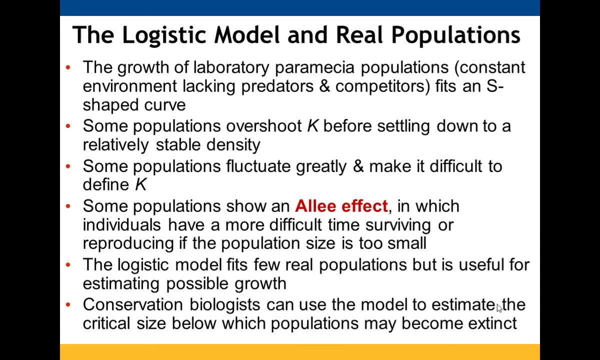 carrying capacity. k value our curve. the number of of individuals in our population starts to. it's still growing, but it's just not. the rate at which it's growing is decreasing. so, um, depending on where your population is, you may see populations that are going to fit more. 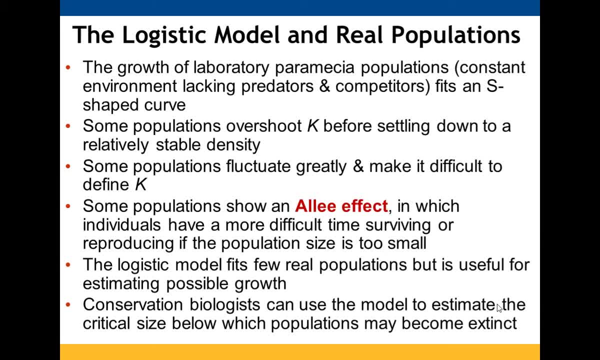 in the j curve or you're going to see ones that might fit more in the s curve. some populations are going to go past the k value and then we'll come back down, and then there are some populations that don't fit um the j of the exponential model or the logistic. 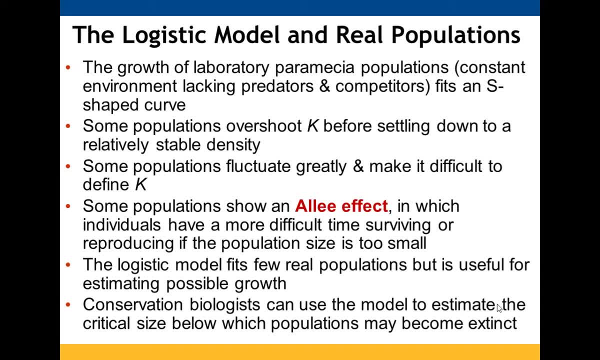 model. and then we have ones that show this alley effect um that aren't able to survive or reproduce very effectively if their size is too small. um. realistically speaking, neither of these models are going to 100 fit populations. um. this model is a little more realistic in terms of 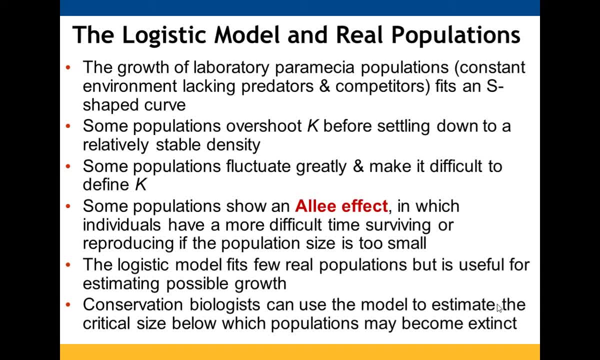 giving us an idea as to whether a population would be able to continue to grow or not. and this is um what one-way conservation biologists are able to estimate. estimate, excuse me, um the size of a population that is needed um before a population would go extinct. so there's your um graphs for the 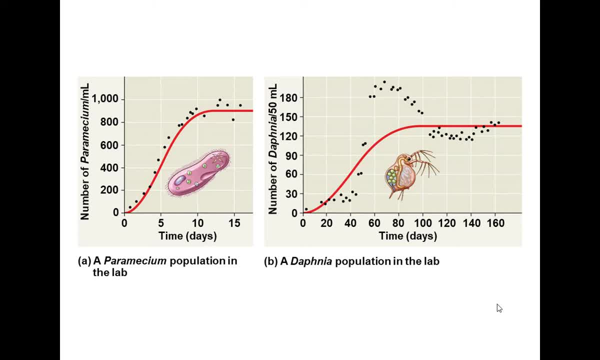 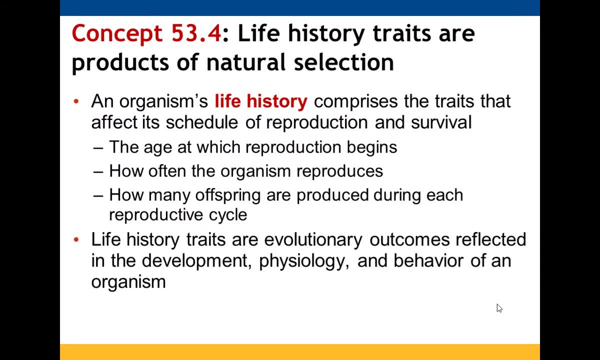 paramecium in the lab and the daphnia. you can see the paramecium falls really closely to that logistic um model, while the daphnia is all over the place. life history, um are the traits that will impact on its being um: ability to reproduce, to schedule a. 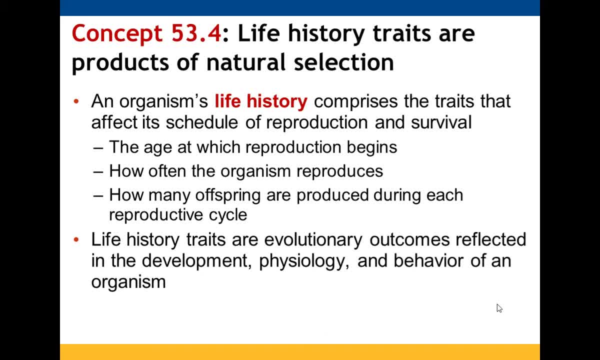 reproduction and its survival. um the factors that will play a role are the age at which reproduction begins, how often it's able to reproduce and the number of off-screen that are produced. um these um traits are. um have an evolutionary basis. um it comes into play with. 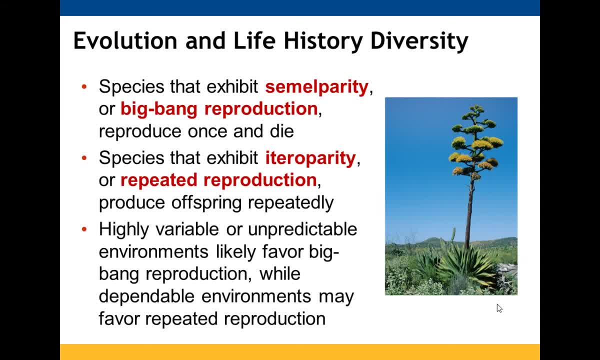 their development, the physiology and the organism's behavior. so there are some species that show semiparity, big bang reproduction- they um are able to reproduce only once and then they pass away. then there are ones that are a terra parity um that are able to repeatedly reproduce. um if you are in an environment that has quite 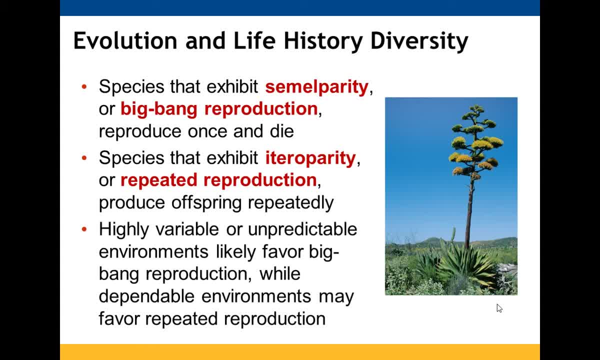 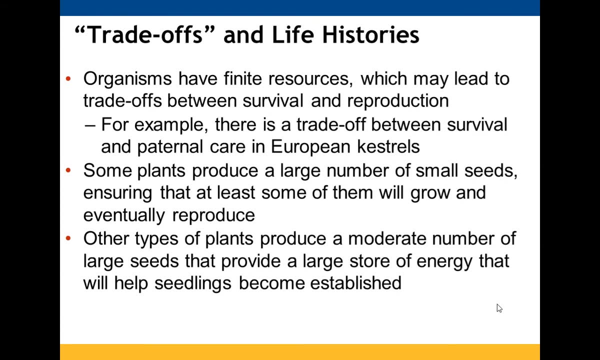 a lot of variables that are undergoing constant change um very unpredictable. your um species is more likely to favor that semiparity, while if your environment is a little more dependable, a little bit more assured, you're more likely to have that species exhibit a terra parity. um other factors that are going to play a role are resources. um, if you only have so much in terms of 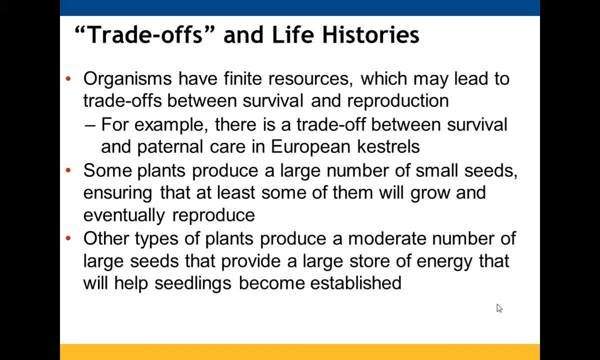 your resources. um, that's going to impact on how you're able to reproduce. so one example we have is with european kestrels. um, there are plants that produce large numbers of small seeds, not expecting all of them to make it. some of them will, though, and then be able to reproduce. then. 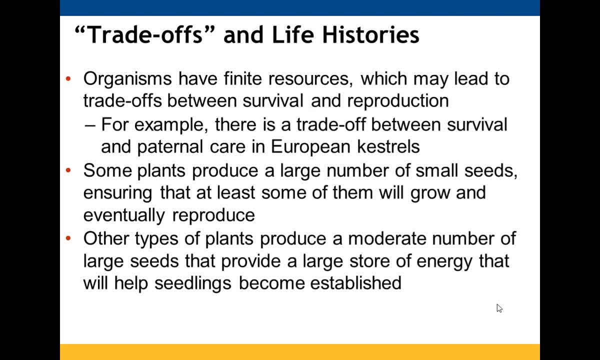 there are plants that don't make nearly as many seeds, and they're not going to be able to reproduce, but they make larger seeds, and so those seeds have more energy, and so a greater number of them should be able to be established as seedlings and to be able to survive. 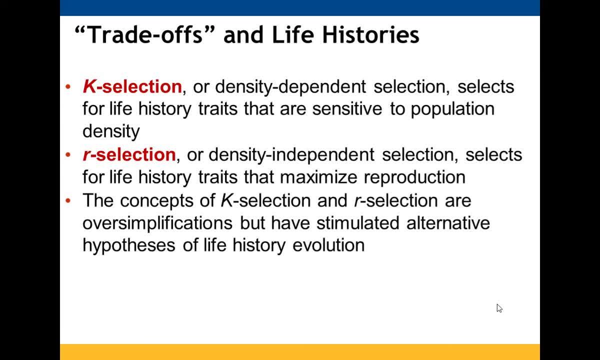 so k selection- density dependent selection is going to take place when the life history traits are sensitive to the size of your population's density. our selection density independent selection is looking for traits that are going to maximize production. um again, these are not absolutes in any way, but it is one way to examine. 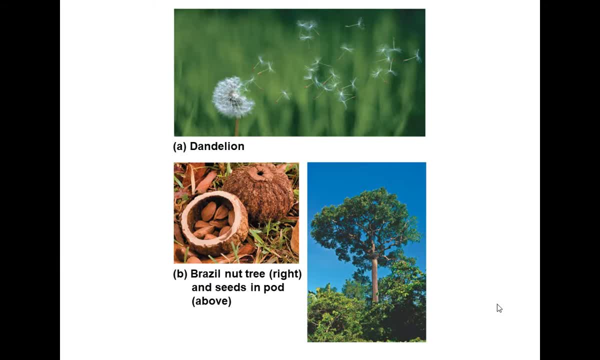 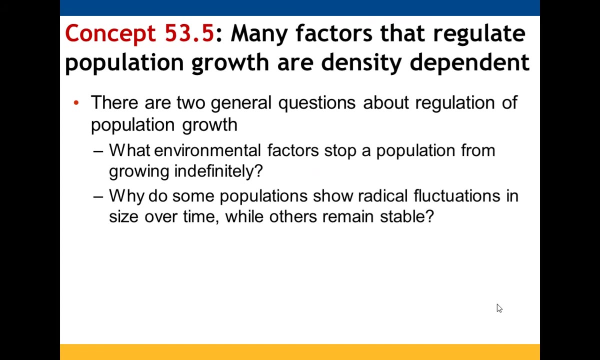 the evolution of life history. so there's a couple of examples of your r selection and then your k selection. factors that regulate population growth tend to be density dependent um. what factors will stop your population from growing indefinitely, and why do you see some populations that have fluctuations while others are able to stay more? 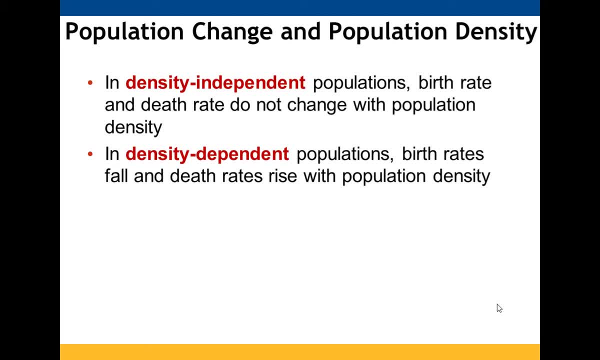 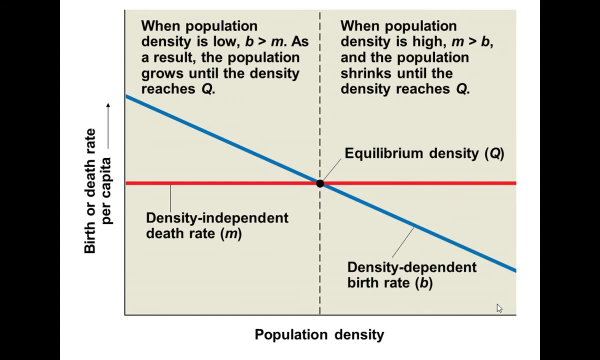 stable. if you are in a density independent population, your density does not affect your birth or death rate. but if you are in a density dependent population, your population density will have a large impact on your birth and your death rates. so, in this particular graph, when you are 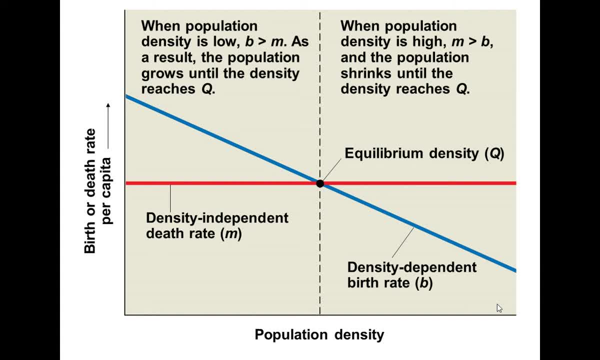 an indensity independent death rate, you're going to stay pretty status quo. you're not dependent on your population density in any way. so that's why you just see the horizontal line. but if you are in a density dependent population, if your population numbers are low, then you're going to have a higher birth. 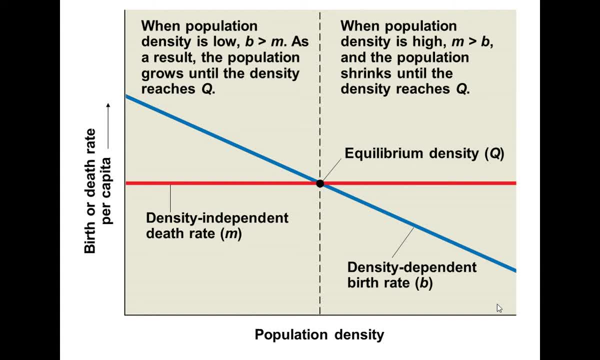 rate than you are. your density, independent death rate and the population will continue to grow. you'll may um more and more individuals will be born and allowed to grow until you reach that equilibrium density. and once you have reached that equilibrium density and you have even more members of your population and you don't necessarily have 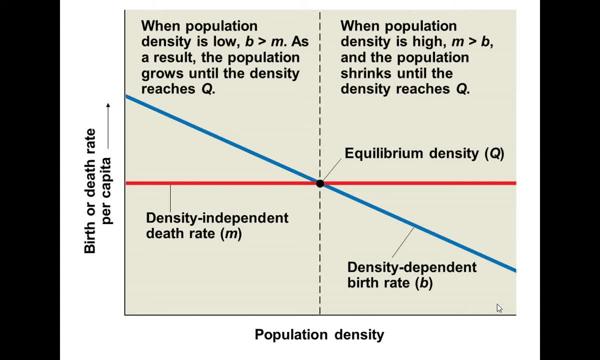 the resources to be able to support them. then you're going to see um that your density independent death rate is going to be greater than your density dependent birth rate and your population is going to shrink um you're going to have more members pass away until you are able to. 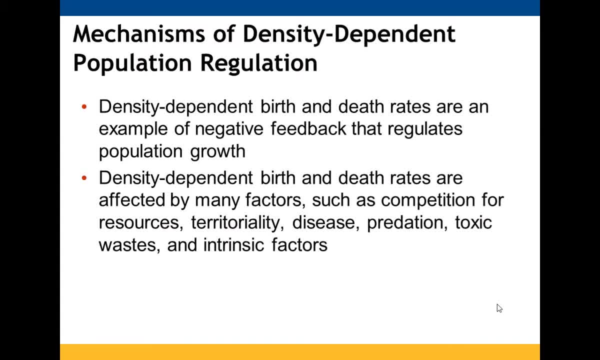 reestablish that equilibrium density- so these are examples of negative feedback- so that your population doesn't get so out of control that now you're fighting for resources and you're not able to continue on with that population. um, so factors that can play a role. um, we talked about resources. 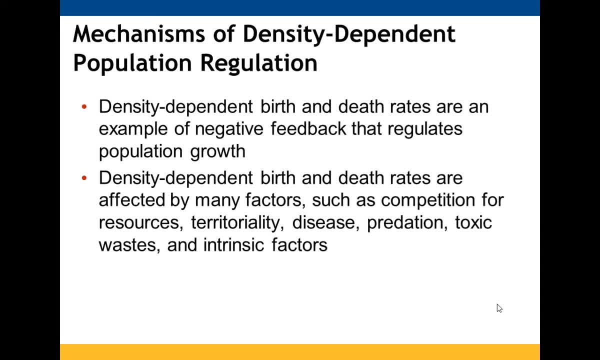 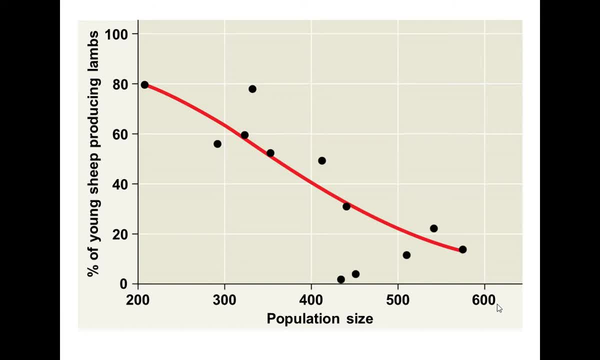 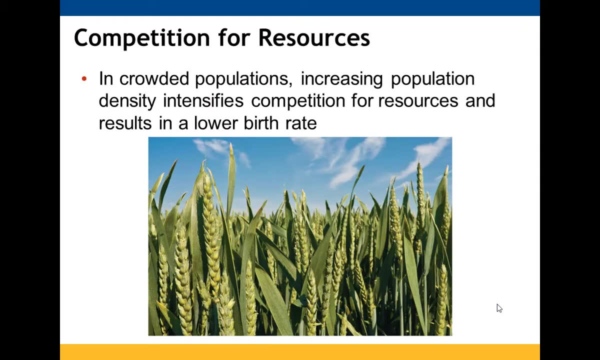 territoriality can play a role: disease predation, toxic waste, intrinsic factors. okay, so there's the issue. we'll go back to the системic right. so let's start in aimiz exceeding and i'm going to highlight a couple problems. um another of these issues is our regrets going to be in our free zosta. 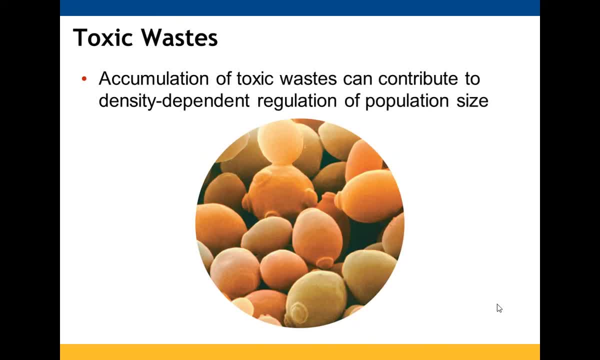 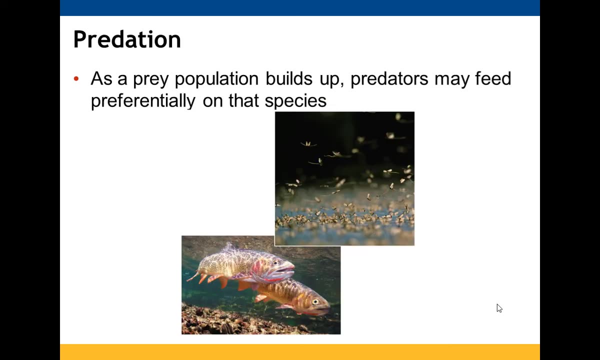 EEEER us. that rate is going to decrease Toxic waste. that can play a role in regulating your population size. Maybe it cuts back on your resources, or maybe it is going to cause your death rates to increase. Predators might feed preferentially on a particular species. that, too, can influence. 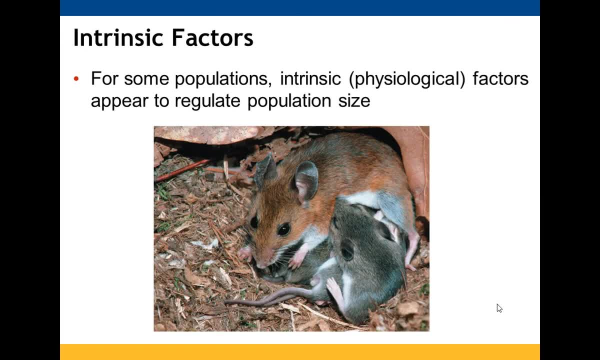 your population, size, Intrinsic factors, physiological. Sometimes mothers have some sort of innate sense that one of their offspring is not going to be able to survive, and so they will cast it off so they can have a better chance of allowing the rest of their offspring to be able. 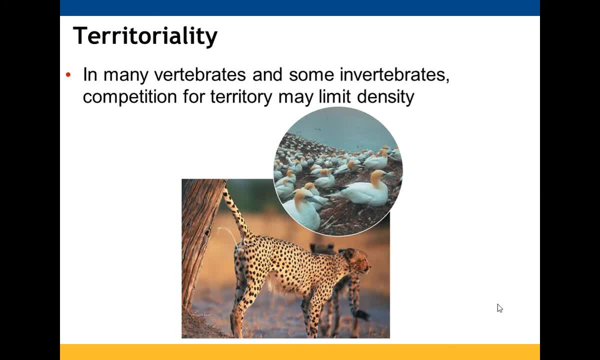 to survive. We talked about territory. Competing for territory could limit your density. If you don't have as much space, you're not going to have as much room for all the individuals. Again, if you have competition for it, it could be predators that are coming in as well. 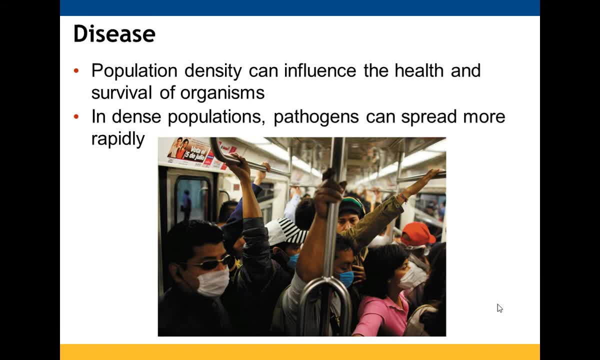 Disease. This is quite timely. Population density can influence the health and survival of your organisms. In dense populations, pathogens can spread more rapidly, and that's what we're seeing right now, unfortunately, with COVID, COVID-19. in areas where there are lots of individuals that are in smaller buildings or 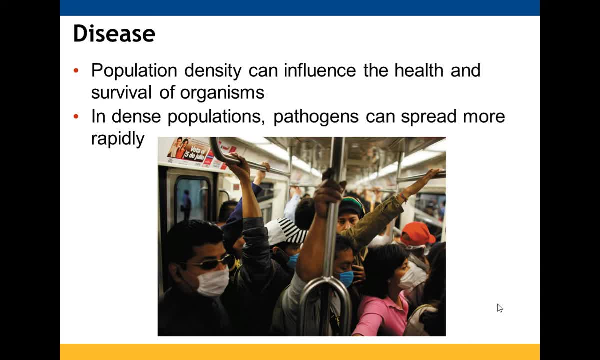 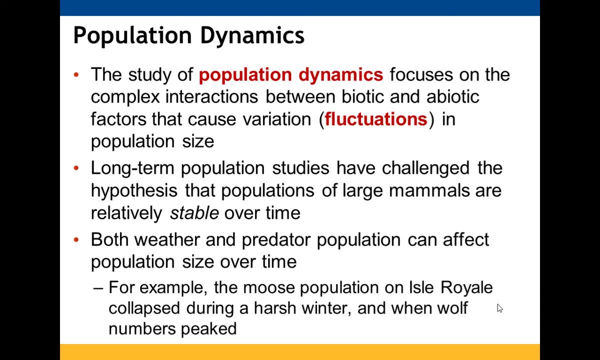 environments, it is making it much easier for that pathogen to be able to spread. Population dynamics is looking at both biotic and abiotic factors that can cause some population size fluctuations. There are more longer-term population studies that have explored the hypothesis that large mammal populations are typically stable and they have 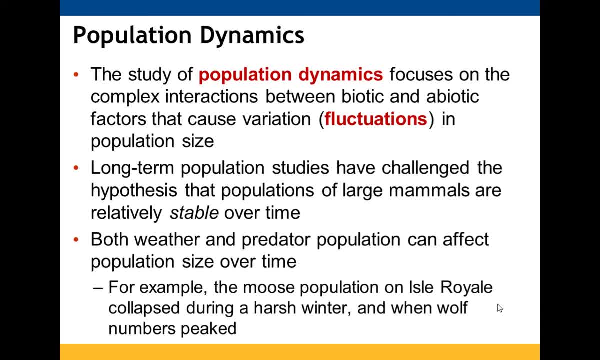 actually challenged those hypotheses. We've seen also that weather and predator population can affect your population size. It's the example you've got here, Isle Royale. There's a moose population there that collapsed during a harsh winter and when that took place, the wolf numbers. 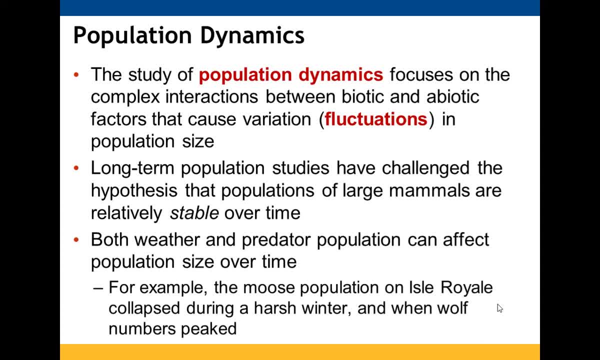 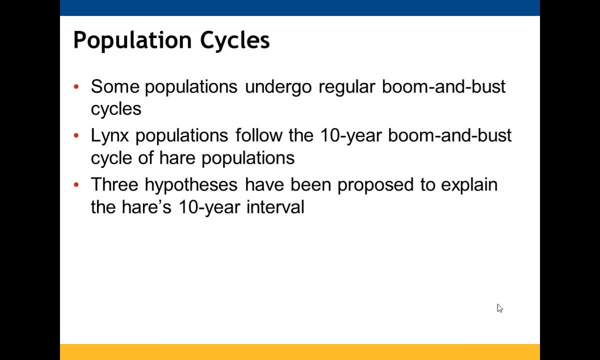 so the moose were their predators- went sky-high Population cycles. Some populations undergo regular boom and bust cycles. We're seeing that right now with cicadas. Lynx populations tend to follow the 10-year boom and bust cycle of hare populations. 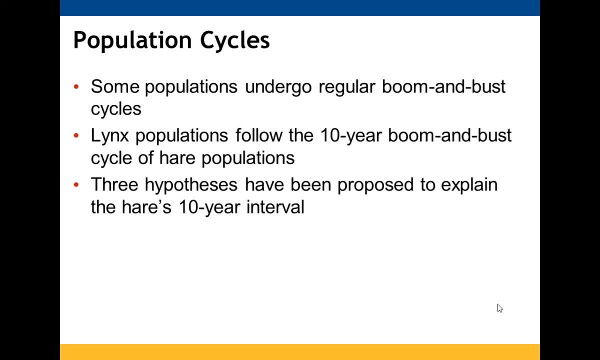 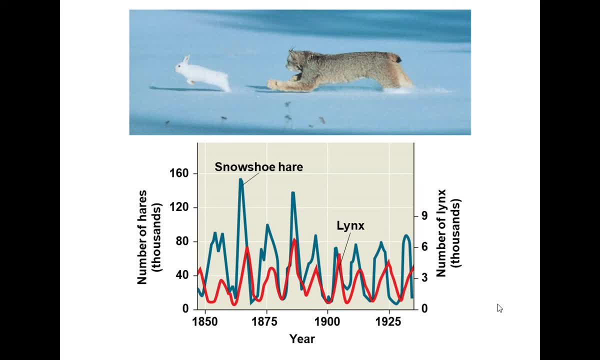 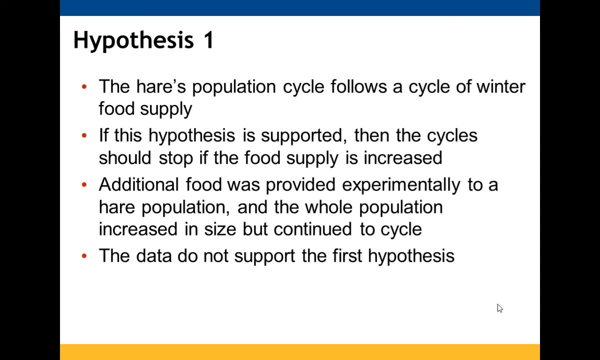 so why might this happen? We're going to look at three hypotheses that would explain that. So there you can see that as the hares increase, so do the Lynx. First one is that the hare population cycle is going to be based on a cycle of winter food supply. 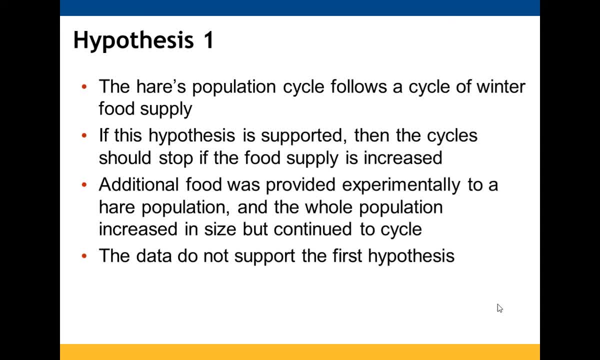 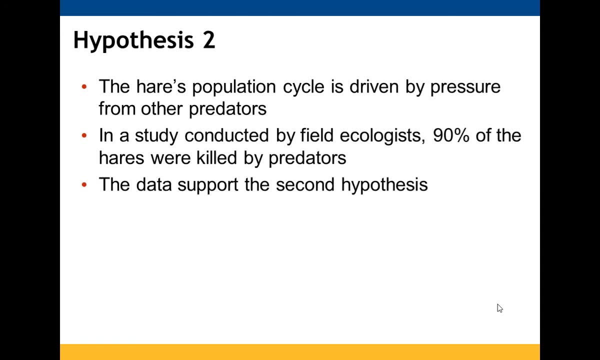 So if you increase your food supplies, you shouldn't see these cycles present, You should see the cycle cease. So food was provided when the population got bigger, but it still continued to cycle. so this hypothesis was not supported And the second cycle, the hare population cycle, was driven. 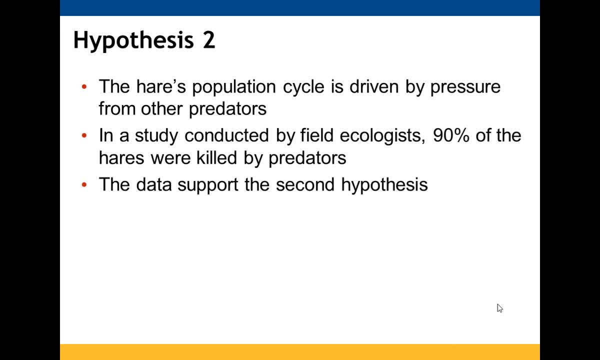 driven, based on predators. So in this study, 90% of the hares were killed by predators. So, as you have more predators, more hares would be needed so that that species could survive. that population Data supported this hypothesis. And then the third one is that it's linked to sunspot. 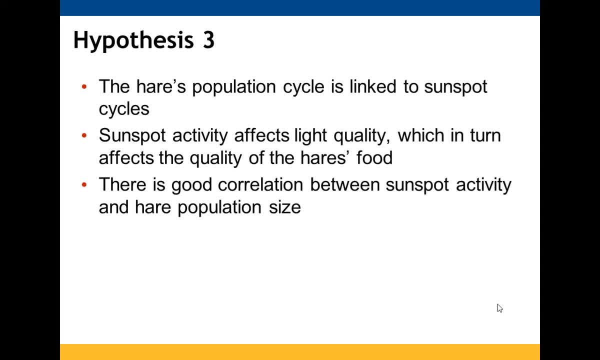 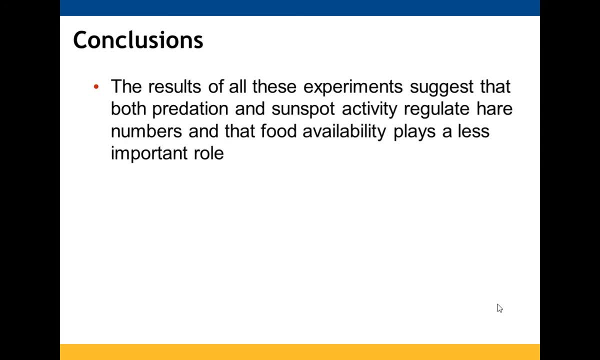 cycles, which is going to affect your light quality, which is going to affect the hare's food, And it's thought that those two might have an influence on the hare's population size. So the results from all three of these different hypotheses that were tested, predation and 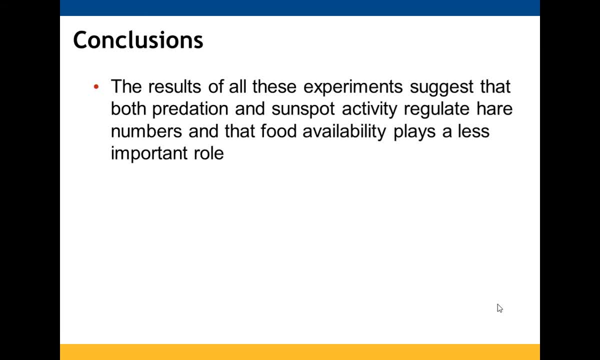 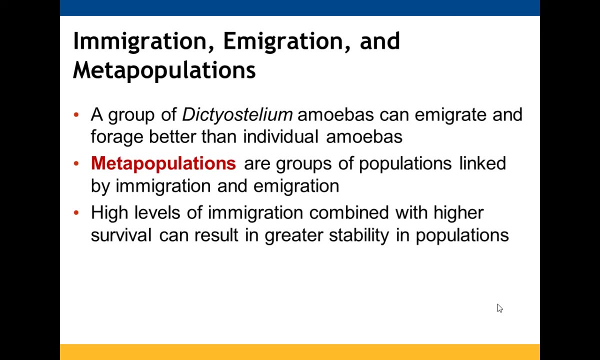 sunspot activity will have influences on the number of individuals that are present in a hare population, but that food availability does not play as big of a role. Immigration: emigration and metapopulations. So this is looking at a group of amoebas that are able to emigrate and forage better than 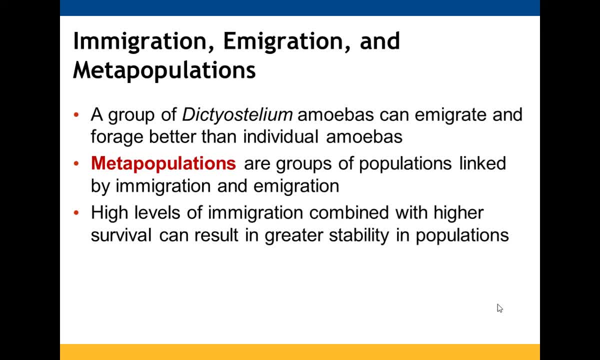 individual ones. So metapopulations are populations that are linked by these two events: emigration and emigration. If you have higher levels of emigration and higher survival rates, your population is more likely to be more stable. Excuse me, The human population. 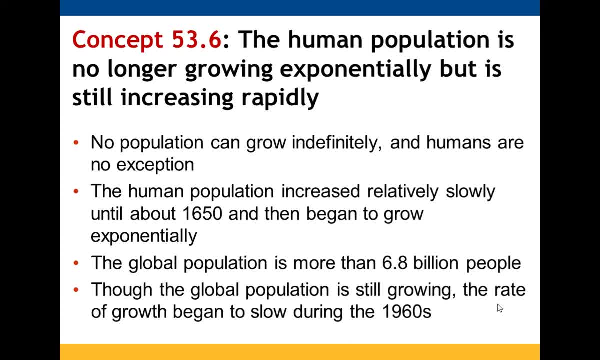 is not growing exponentially anymore, but it is still increasing. We are limited by the resources and all those other factors we talked about. It was growing fairly slowly until about 1650, and then it started growing exponentially. But our rate of growth has slown down in the past 50 years. 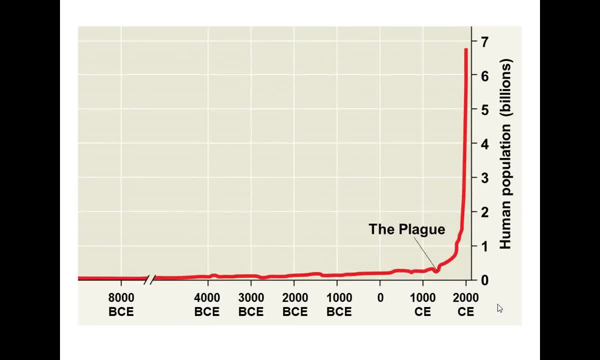 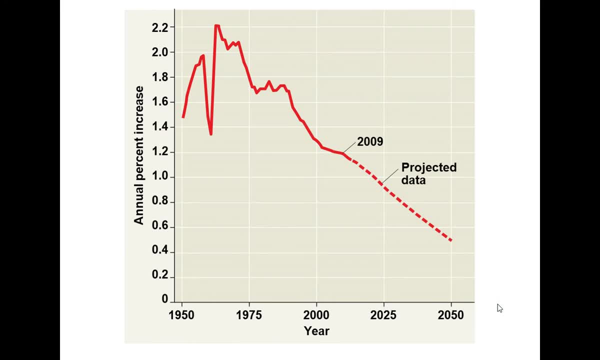 Okay. So again this first one. you got BCE, you got the plague in there, and then you see the huge skyrocket in population, And even within that skyrocket, though, you can still see that, although we are having increases, our increases are diminishing. To maintain: 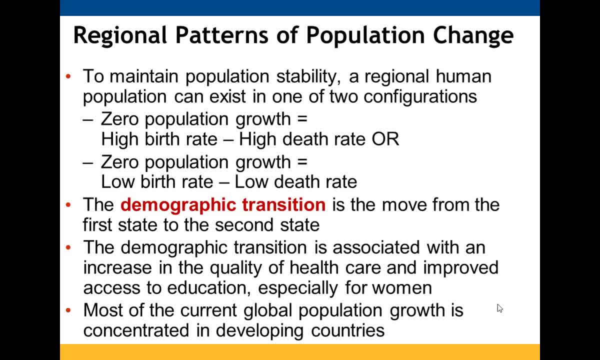 population stability. human populations are going to exist in either of these two configurations. You're either going to have zero population growth because you have both a high birth rate and a high death rate, or because you have a low birth rate and a high death rate, or 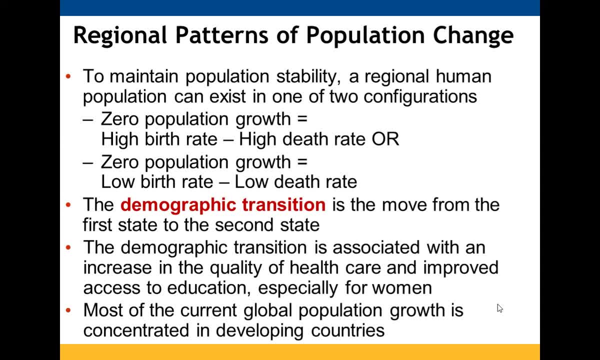 because you have a low birth rate and a low death rate. A demographic transition is when you move from the first one, where they're both high, to the second one, where they're both low. This is going to happen when you are in areas where healthcare quality is sound. 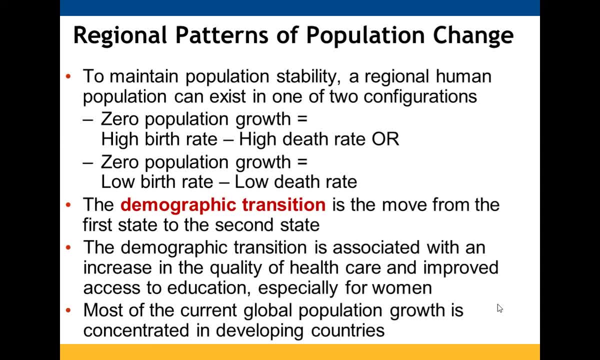 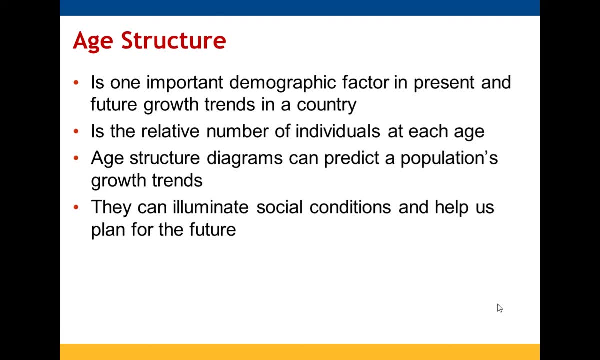 improved educational access, especially for women. What we're seeing is that the global population growth is concentrated more now in your population than it was in the past. So developing countries, So age structure will play a role in examining what growth trends are. 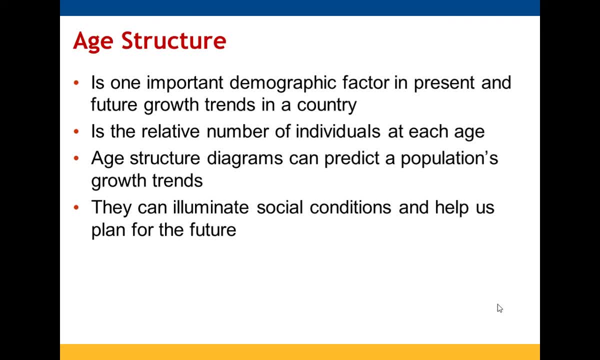 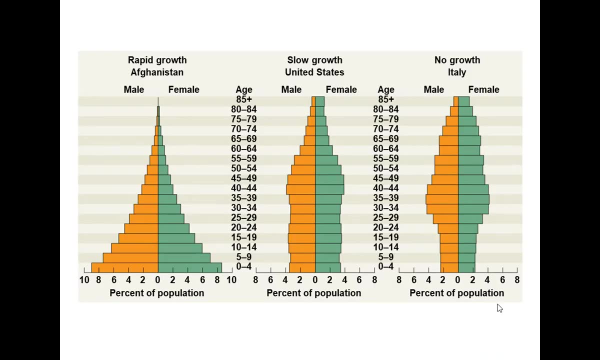 looking like in a country, how many individuals, relatively speaking, are present at each age, for both males and females, And this can kind of help to predict future growth trends. It also gives us a better idea of social conditions and being able to plan for future events. So with this first one, 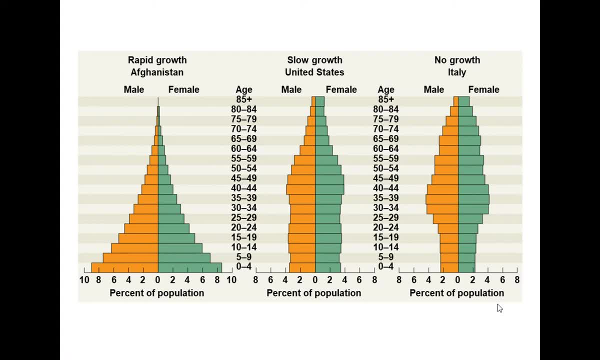 we see with Afghanistan. we see they're having rapid growth- lots of younger children, zero to four at the bottom. So this would be an example of a pyramid. And so because we are having way more individuals at the younger ages as opposed to at the older. 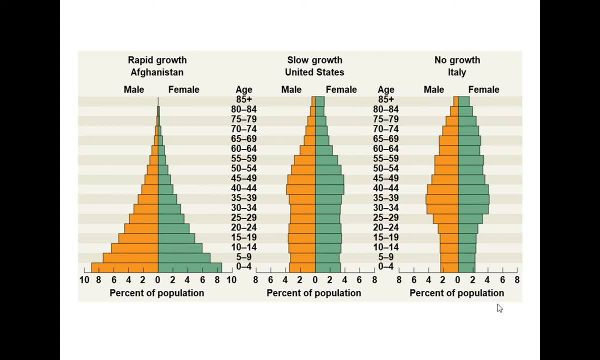 ages, we are having exponential growth take place. in this particular example, In the United States, we're undergoing slow growth. We have a stable population. We have what we refer to more as a bell-shaped population where, relatively speaking, if you look down from zero to four up to you know into your 50s- I'm not saying it doesn't- 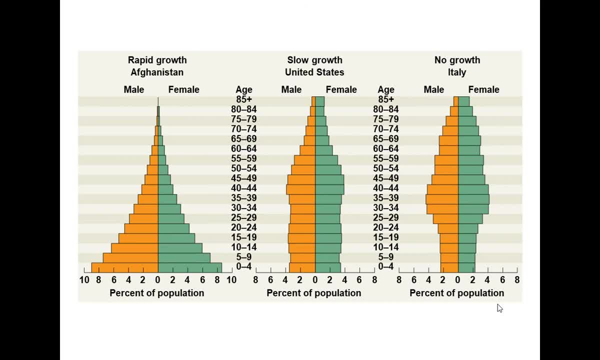 vary a little bit, but it's pretty consistent across the board. And then after you get through the 50s- remember we talked about the type one survivorship curve- that as the age of the individuals in that population increased, we saw a greater number of deaths as that age increased. And that's what you're seeing happen. 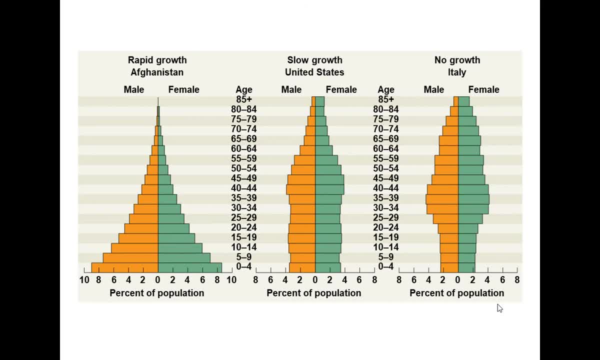 after you get out of the 60s or out of the 50s, But it still takes quite a bit to get there. Whereas with Italy we're not seeing a whole lot of growth, This curve is representing more of an urn shape. If you look at the bottom, you see that they are having much fewer the number of births. 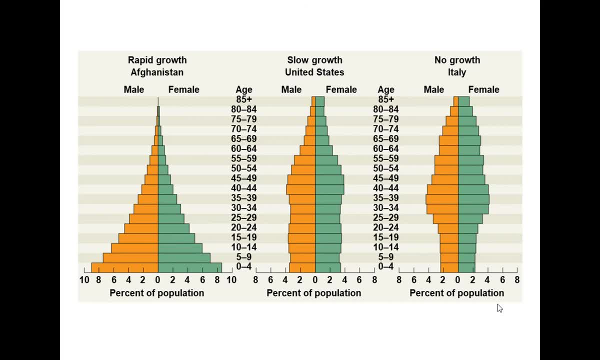 is much smaller compared to what we saw with the rapid growth and the slow growth And that number is saying small. And then as you get up into your middle ages- 30s, 40s, 50s- we have a greater number of individuals in the population at those. 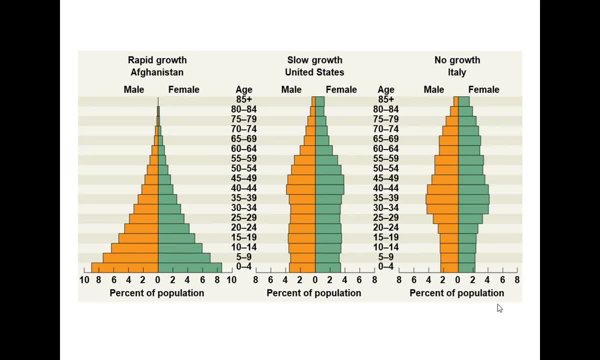 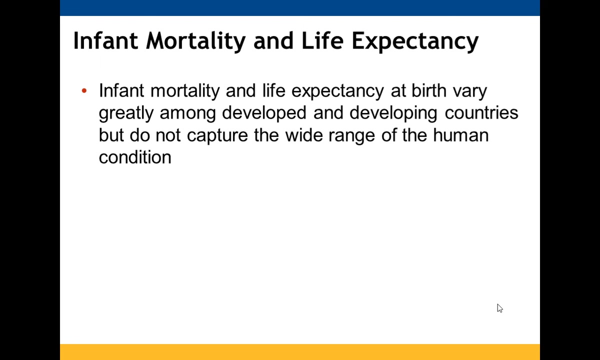 middle ages, And then we're seeing it substantially decrease, but not to the numbers that we saw with the rapid and slow growth. So when your birth rate is falling below your death rate, you are typically seeing what we call a declining population Infant mortality. life expectancy will also play roles. These are going to vary depending on what 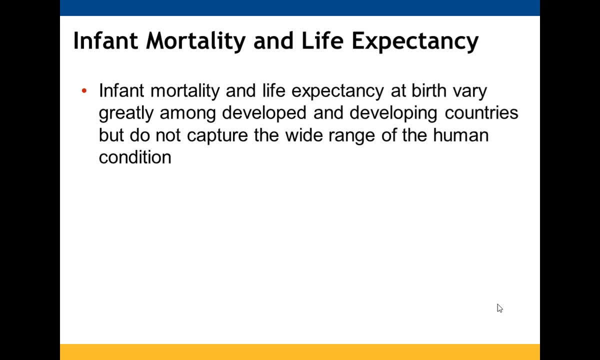 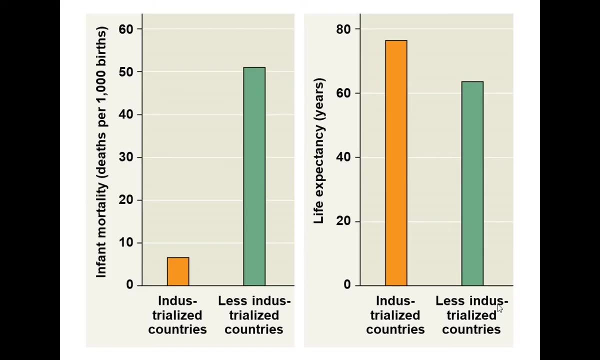 resources are available to you in your country. They are not. they're a snapshot and they are not an absolute. the only figure you should look at to examine what's taking place with the human condition in a given country. So in your industrialized countries, we see that 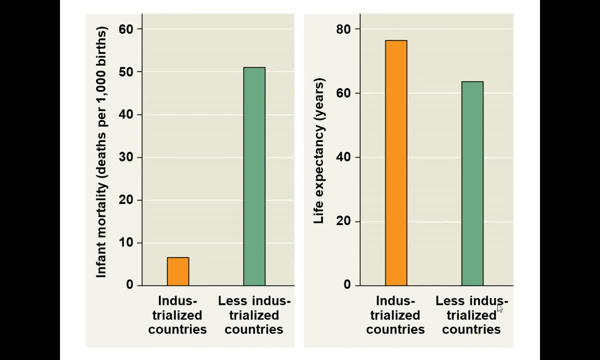 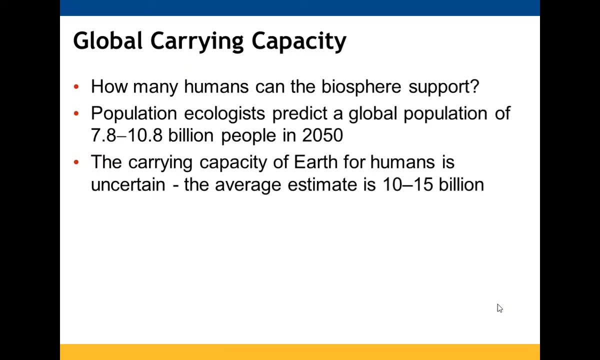 in fact, in the United States, we see that the number of births that are available to you in your infant mortality rates are low and life expectancy rates are high as opposed to the less industrialized countries. So how many humans can be supported by our biosphere, the global carrying? 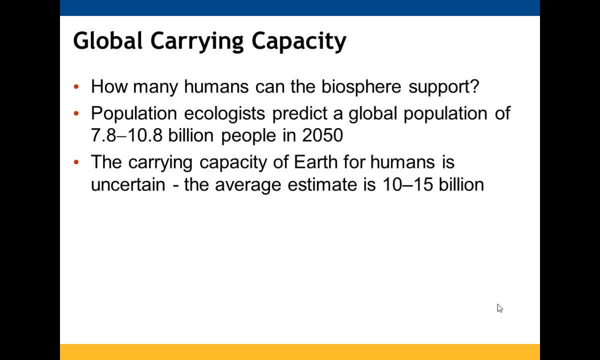 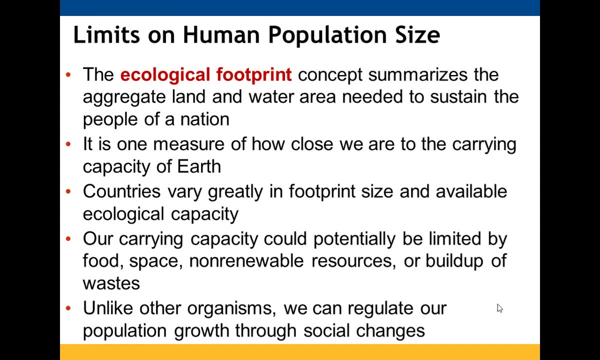 capacity. Population: ecologists expect that we should be able to hold approximately 8 to 11 billion people in 2050.. What exactly the carrying capacity is on the earth for humans is not known, but it's estimated. So ecological footprint: this concept is basically giving us an idea as to what land and water